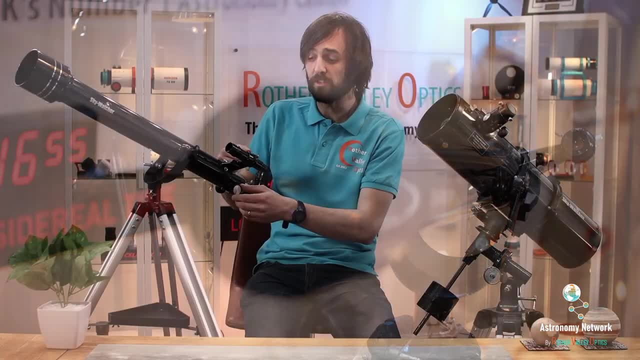 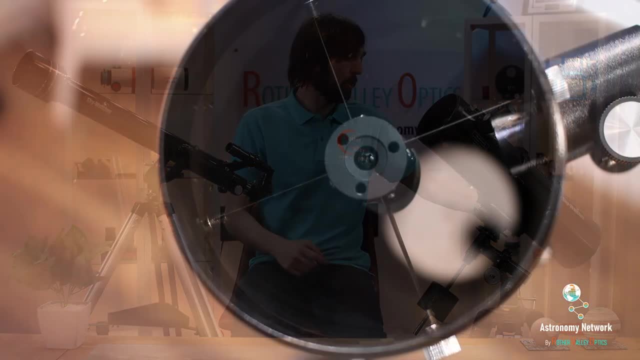 all the way down through the scope in one direction and is focused to a point at the back, which is where you focus it, to your eye now, with a reflector. light still comes in through the front, but it passes down. the scope is reflected back by what's called your primary mirror and then it is reflected. 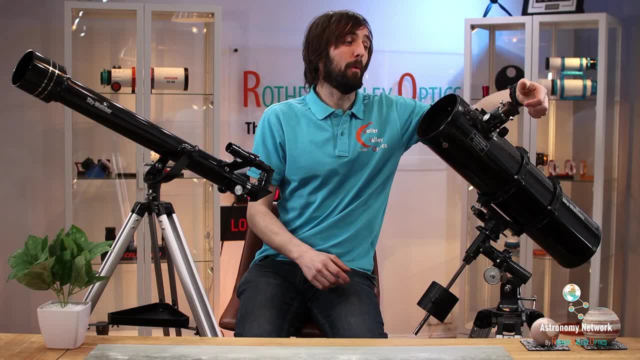 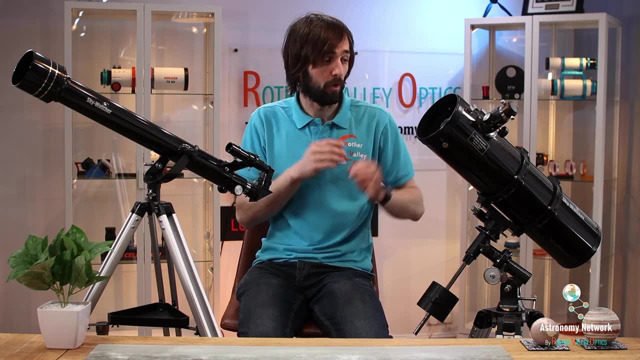 again by the secondary mirror to your eye, which you just pop the eyepiece in there and it comes out the side. now what that means is, when you're using it is, with a refractor you look down and up through the telescope, whereas with a reflector you're looking in from the side and you're looking down at a reflected. 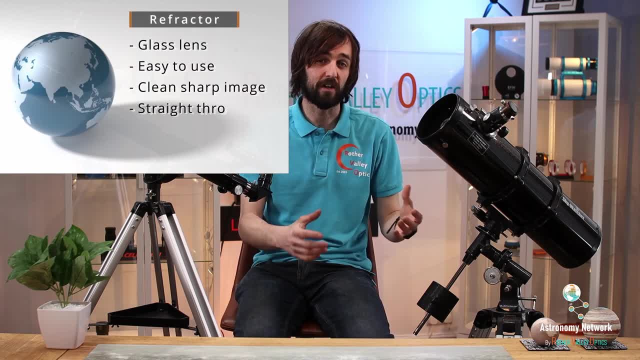 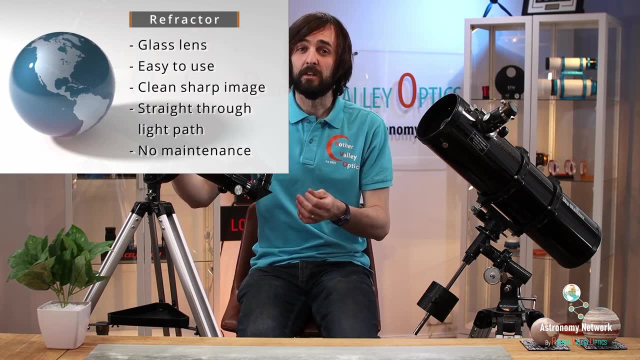 image. another thing to bear in mind when choosing a refractor or a reflector is how much maintenance you're prepared to do. with a refractor, they're pretty much maintenance free. they're a sealed lens. there's no reason to collimate it. there's all you need to do is keep it clean, whereas with 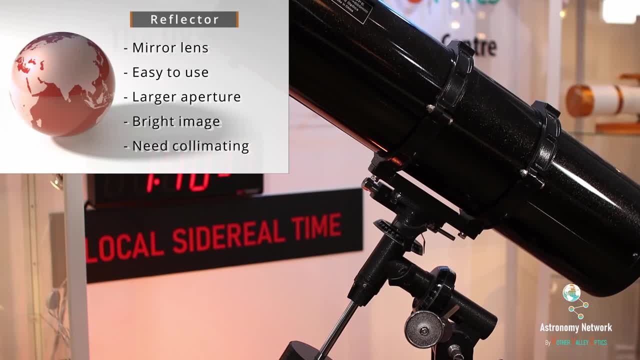 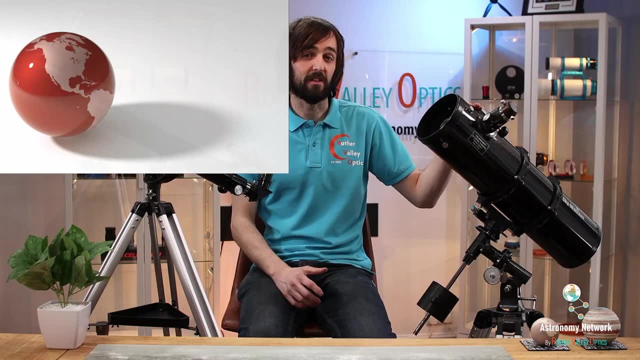 the reflector. the mirrors can move slightly, so you will need to collimate it periodically. now i'm not going to go over collimation in this video, i'll save that for another one. but that's one thing to bear in mind if you are choosing a reflector that you will need to. 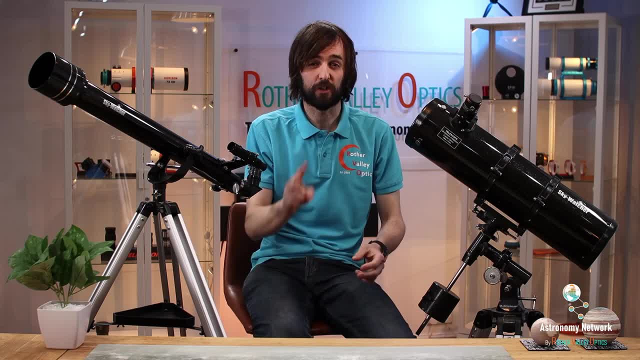 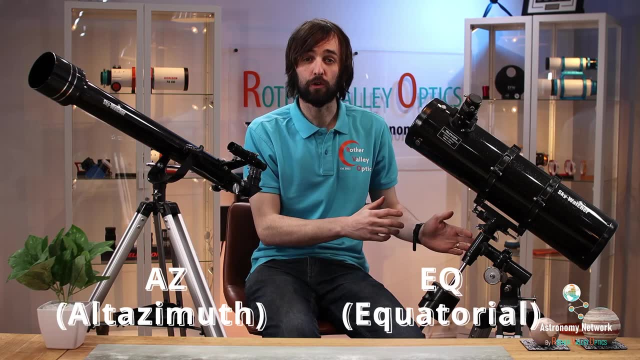 collimate it at some point. so next we have the types of mounts. there are two main types. there's the az and the eq, but the az is short for alt azimuth and the eq is short for equatorial. so, starting with the alt azimuth, these are very simple. they just move up down, left and right. 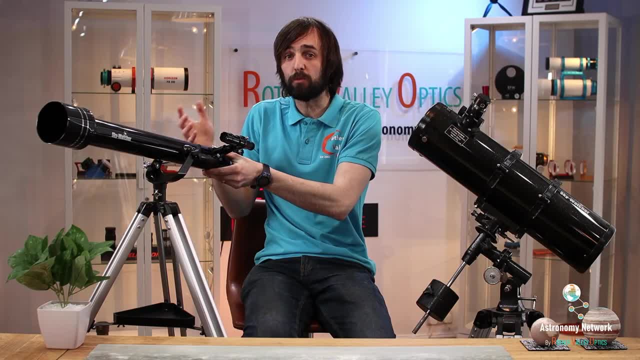 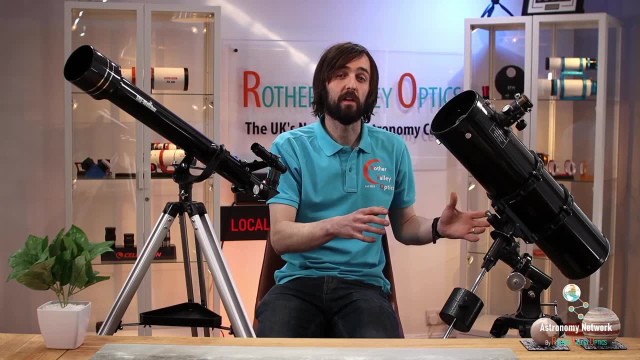 in altitude and azimuth. so when you're looking for an object in the sky you simply just move it around and scan the sky like that, whereas with the equatorial they move in a different way. they move in what's called right ascension, and that's when you're looking for an object in the sky. 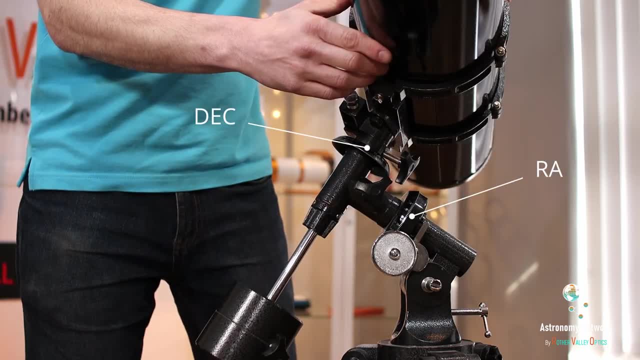 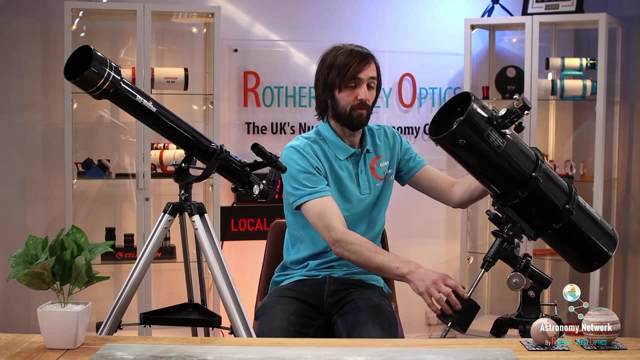 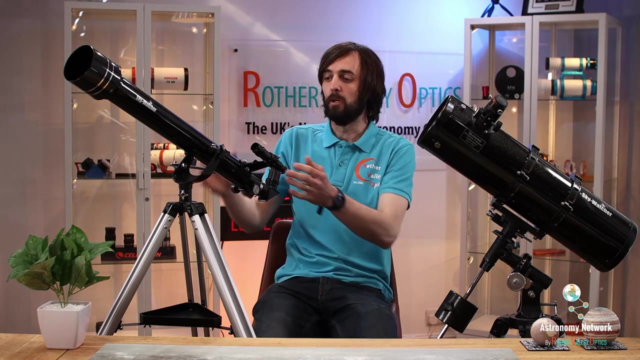 ascension or ra, and dec or declination. so your ra is this movement here and your declination is your left and right. which is this movement here? now, what that actually means is when you're following an object, you do it in different ways. with the alt azimuth mount if you're trying to say follow a planet, if you're, 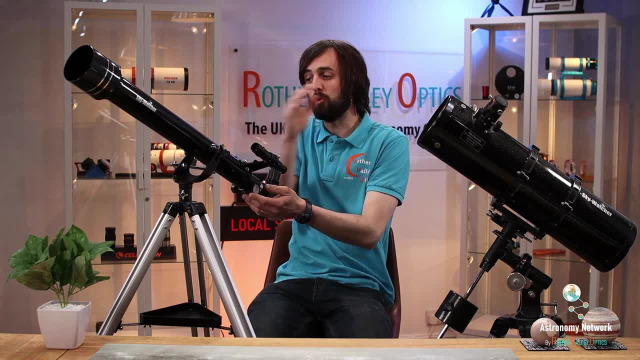 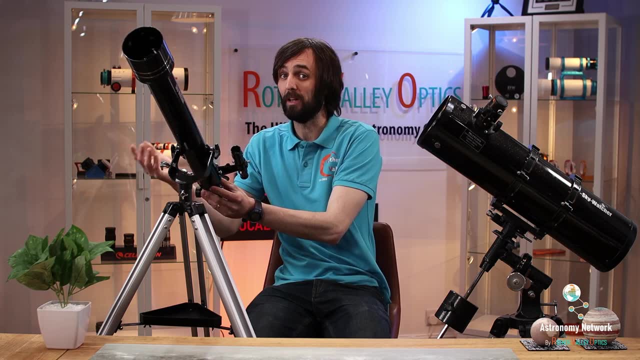 looking at jupiter. you're going to need to follow it across the sky as it moves. you're going to need to do that in two steps. with the alt azimuth. you're going to have to go across and up, across and up, a little bit like that as it moves around the sky. now, with the equatorial mount, 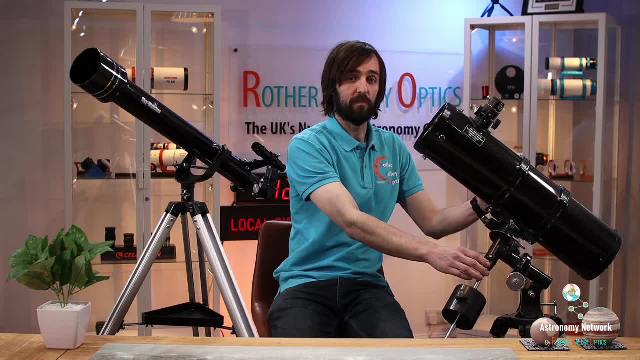 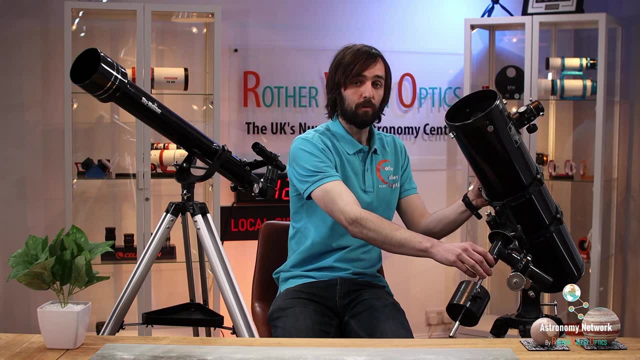 once you have set it up, you actually only need to follow it with the right ascension. so you move your declination to find the object. once you've found it, you move the ra and it will follow it across the sky in one movement. now one thing to bear in mind when choosing one of these. 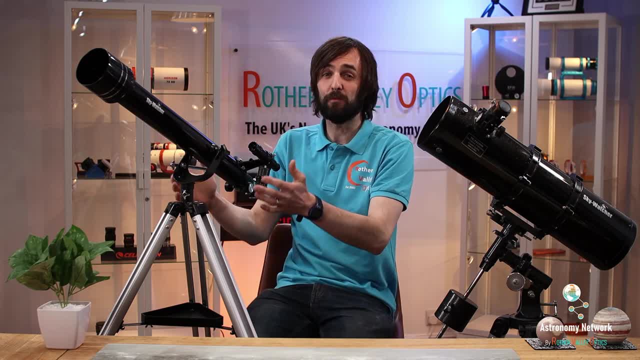 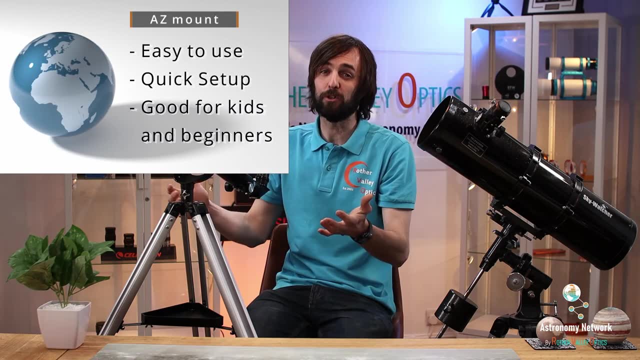 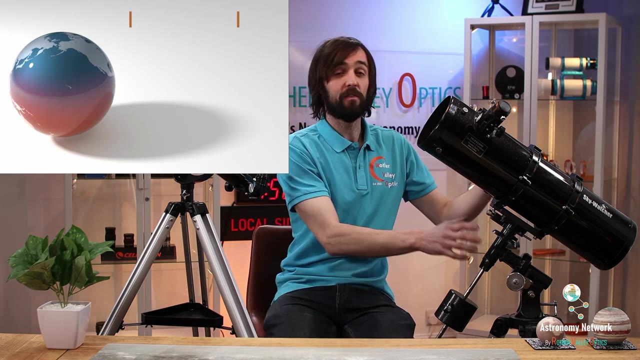 two mounts is how easy they are to set up. the alt azimuth is by far the easier one to use. you simply just extend your tripod legs, you pop your telescope on top and you're pretty much good to go. so they're very good for children. they're very good for beginners, because there's no complicated setup now with an equatorial mount. 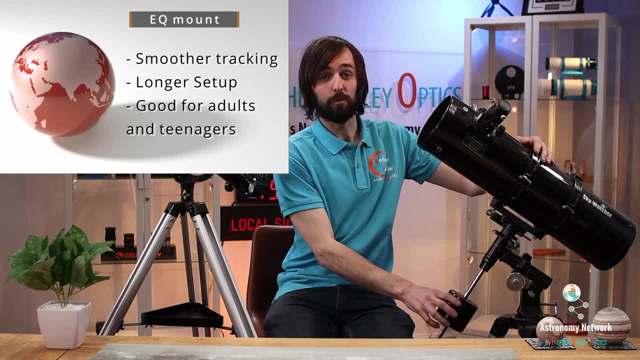 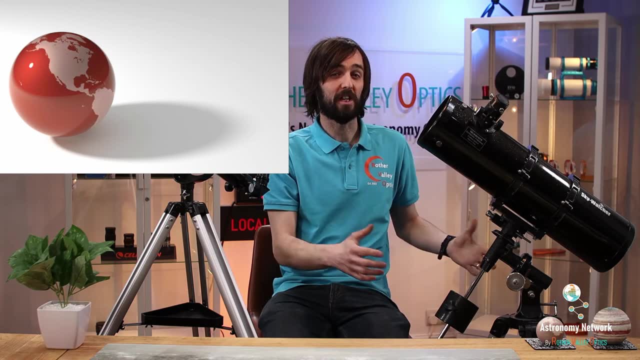 there is a little bit more involved. for a start, you need to set up your counterweights, and you also need to do something called a polar alignment. now i'm not going to get into all the ins and outs of how to set up an equatorial mount, because that will be a whole other video. 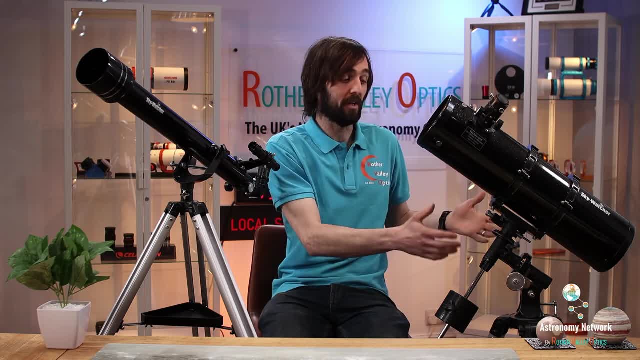 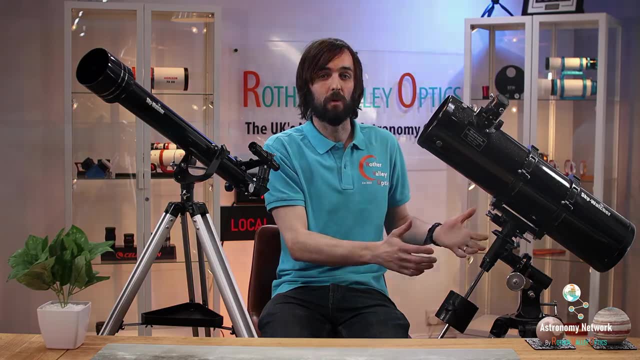 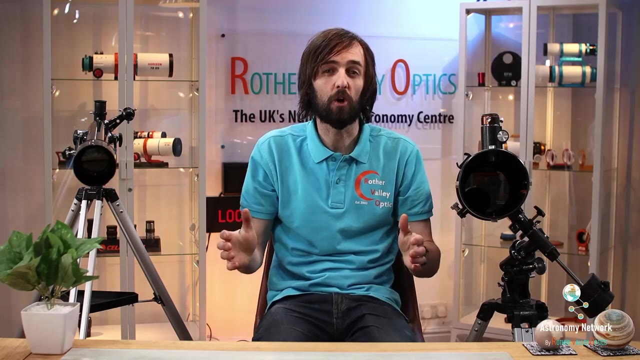 but there's one thing to bear in mind: that if you are buying this type of scope on this mount, then it's going to maybe be better for, say, a teenager or an adult, because there is a little bit more setup involved. okay, so, moving on, we're now going to get into some of the terminology surrounding telescopes. 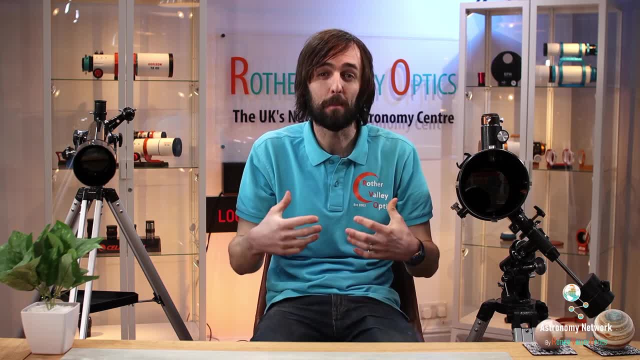 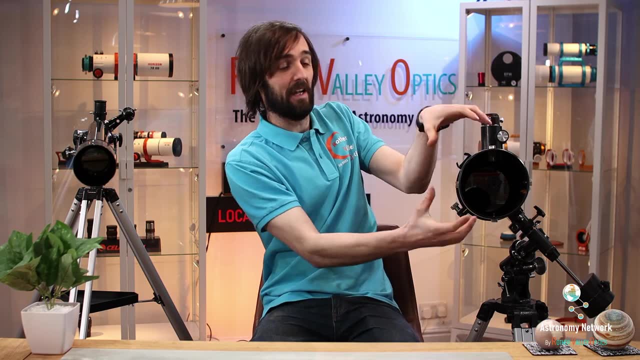 and the main ones are aperture and focal length. now, in my opinion, these two things are what are going to be very important when choosing your scope now. the aperture, put simply, is the diameter of the actual telescope if you look at the reflector here. if you were to measure the mirror at the back, it's 130 millimeters in aperture. now. if you look at this refractor, if you was to measure the front of this lens, this one's only 60 millimeters in aperture. now. what that actually means, obviously, is that this is a bigger scope. it's a wider scope, it's going to get a lot more light in. 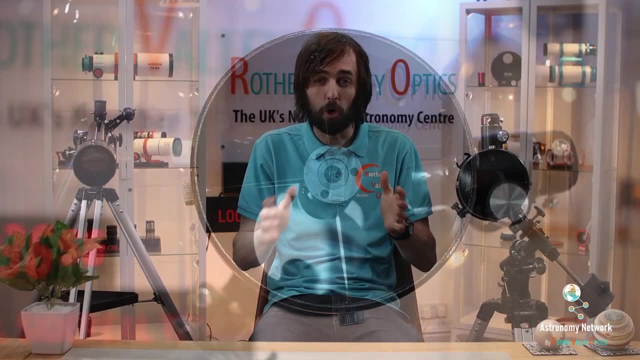 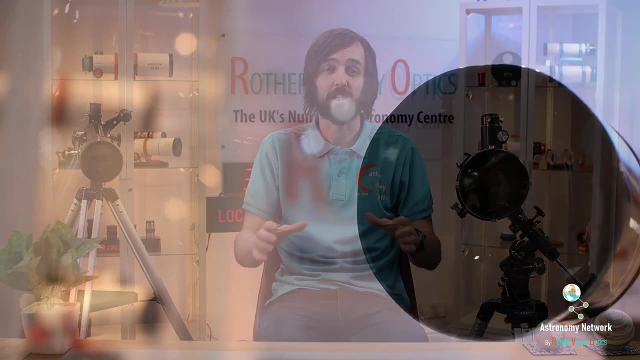 now more light. it means more resolution. you will see more objects and you will get better definition overall. so by having that bigger aperture, you've got a better chance of seeing more objects in the sky, which is what it's all about. so i would say, above all else, when choosing your 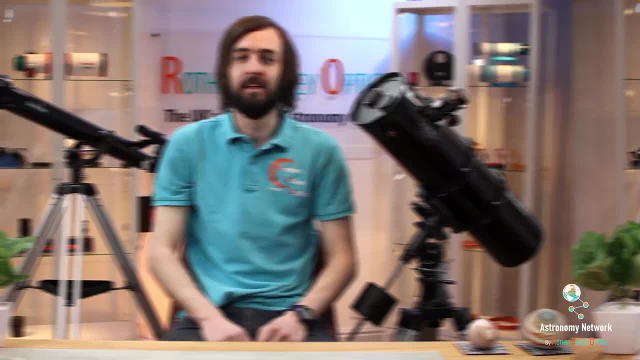 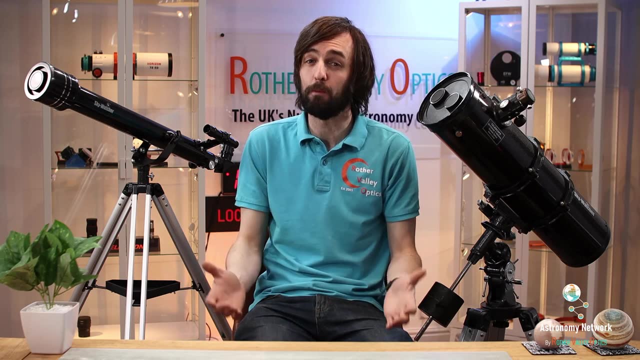 first telescope, try and go for as big an aperture as possible. so it's not all about aperture. you also want to consider something else, and that is focal length. now, the focal length determines how much magnification you're going to get out of the telescope. now, focal length is measured from the 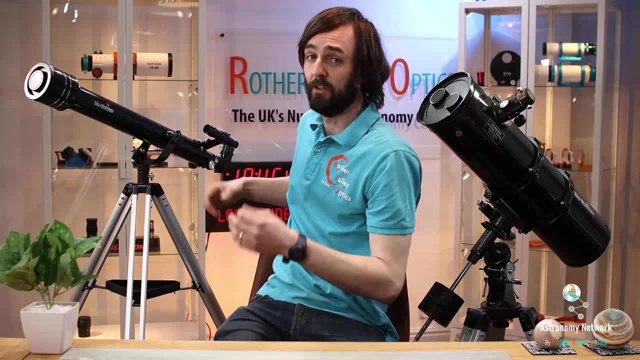 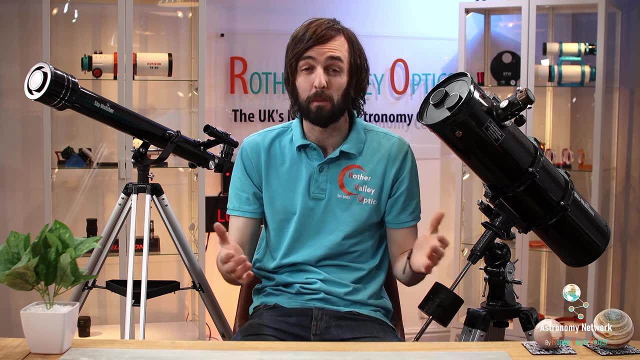 main optic to the point at which the light is focused, and the longer that focal length, the more power you've got. more power means more magnification. now that's important if you're say wanting to look at planets, because you need quite a long focal length for the planets. 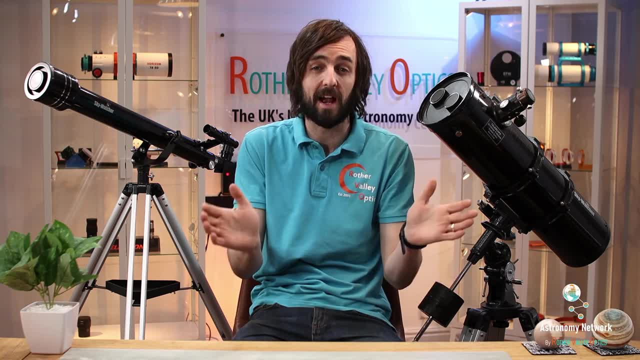 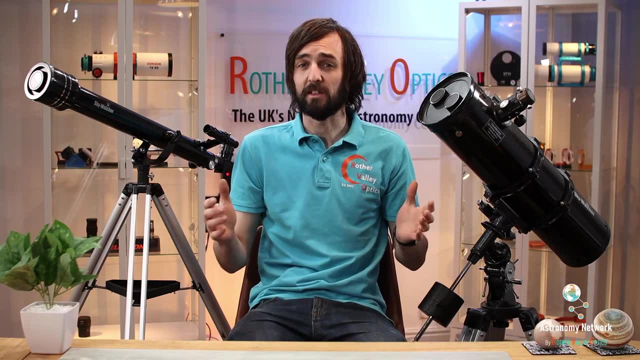 whereas if you're wanting to look at, say, in a wider area of the sky, something like andromeda or orion nebula, then you'll want a shorter focal length. now these two scopes are actually quite similar in focal length. this one's 650 mil and this one is 700 mil, so you're not going to notice. 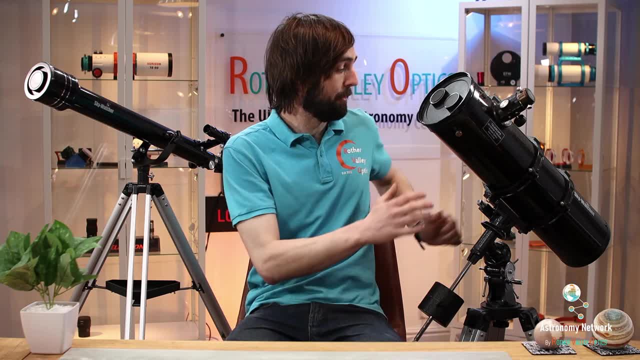 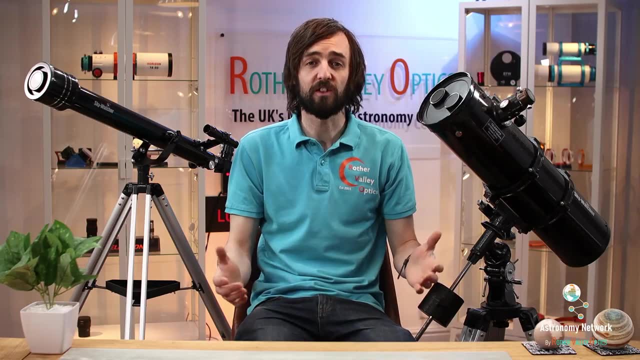 a massive difference in the amount of magnification between them. however, because this has the bigger aperture, like what i mentioned before, you will get a brighter image at that same magnification. so both reflectors and refractors come in various different focal lengths. now this particular telescope is called the explorer 130p. 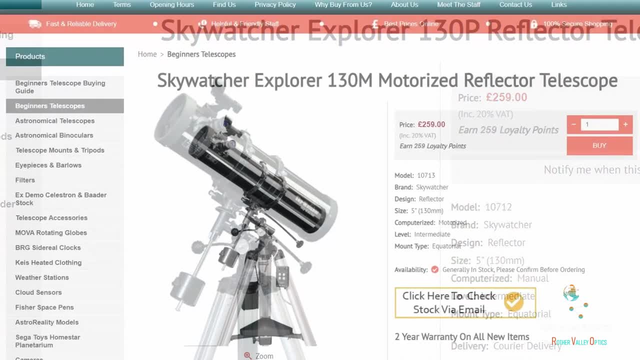 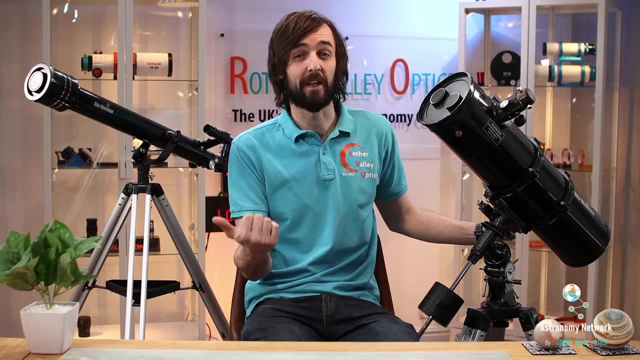 and it has a 650 millimeter focal length, but you can also purchase this with a 900 mil focal length and that's called the explorer 130 eq2 and the explorer 130m, and i'll be getting onto those a little bit later on. and finally, the magnification of your telescope. it isn't just determined by your 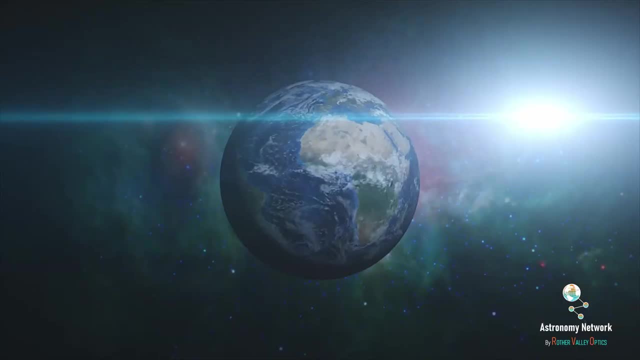 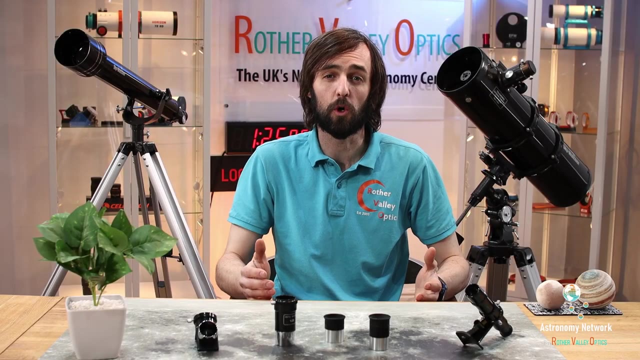 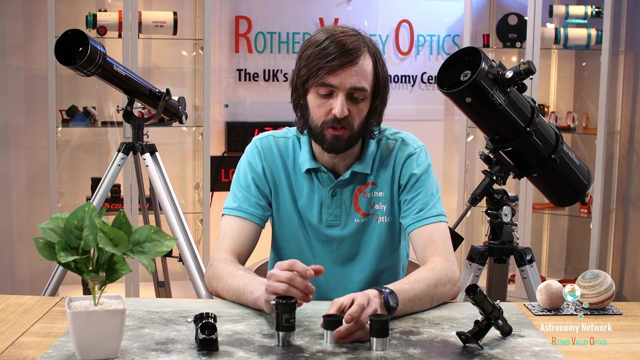 focal length. it also depends on what eyepiece you're using. so now i'm going to talk about what accessories come with your telescope and what i would recommend you upgrade or maybe add on in the future. now, pretty much every telescope package- most beginner packages- will always come with at least two eyepieces. one will be. 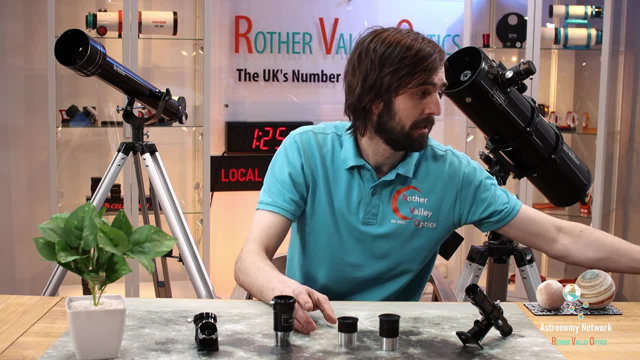 a 10 millimeter and the other will be a 20 millimeter. now, on some packages you'll also get a balo lens as well in the box. you'll also get a finder scope. now this one is a optical lens, so we're going to be doing a little bit of our look at this one ever somar. 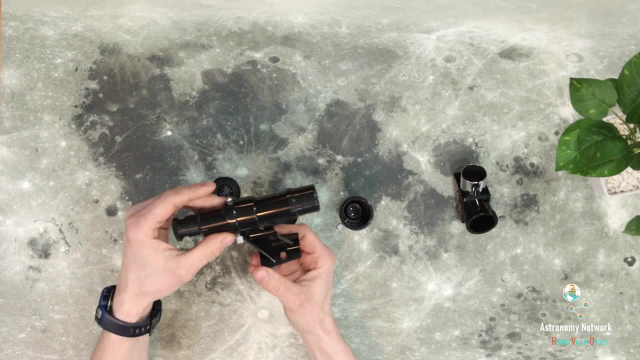 on tele. Hahahahaha, this other one is a hop piec. and then, of course, if you're in your phone, you'll have to do some of the controlled setup. you'll need to do that as well. all the cameras, you've seen them all on there. they're all there. 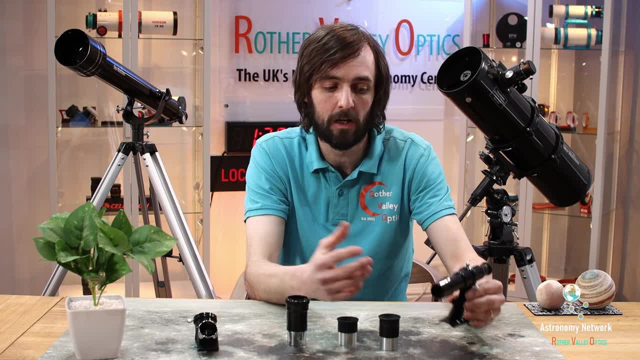 they've all filled up. now I'll just say for the rest of today's video: so if you want the measures, you'll need a optical finder, but sometimes you'll get a red dot and you'll also get a diagonal if you buy a refractor but on the reflector you don't get a diagonal. 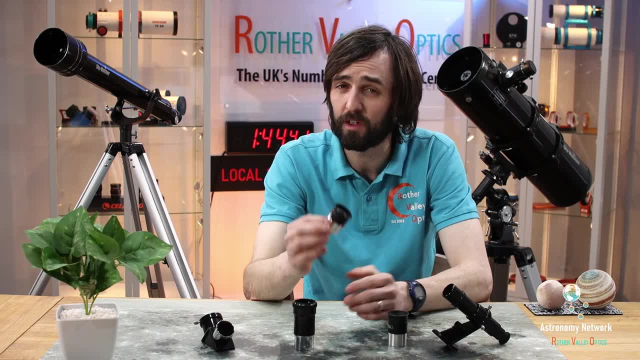 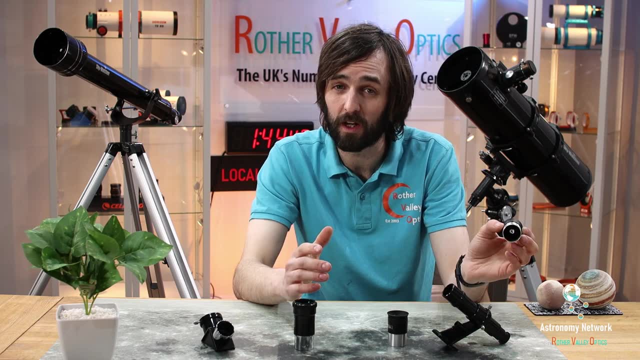 because they're not needed. so I would pay close attention to the eyepieces, because that is going to determine how much magnification you're going to get. now, to work out the magnification, you take the focal length and divide that by the focal length of the eyepiece. now, if we look at the reflector, which was 650, 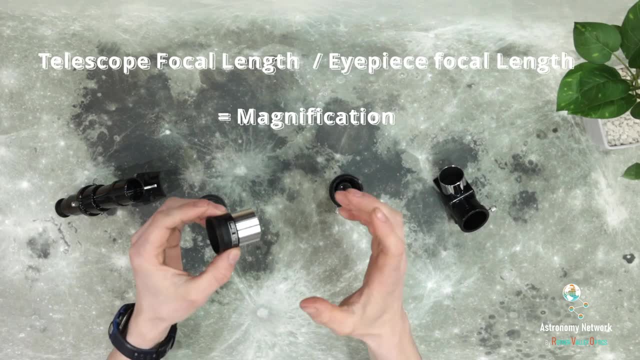 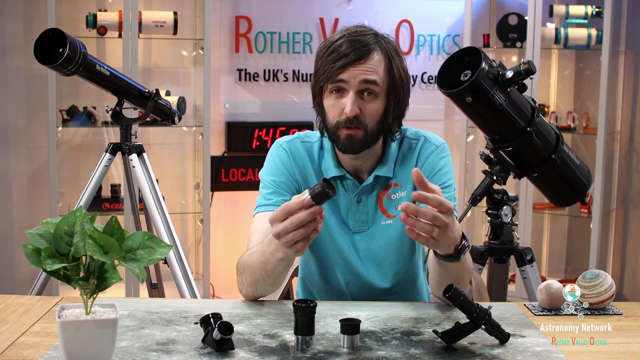 mil. if you divide that by 10 millimeter, that gives you the magnification which is 65 times. so if you was to then put in the 20 millimeter, that's going to get you a lot lower power. it's going to be just over 32 times magnification. so what? 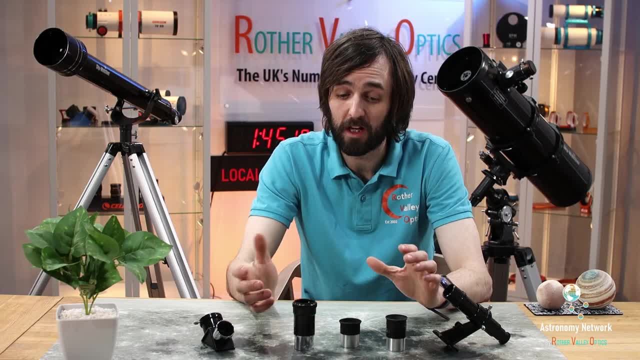 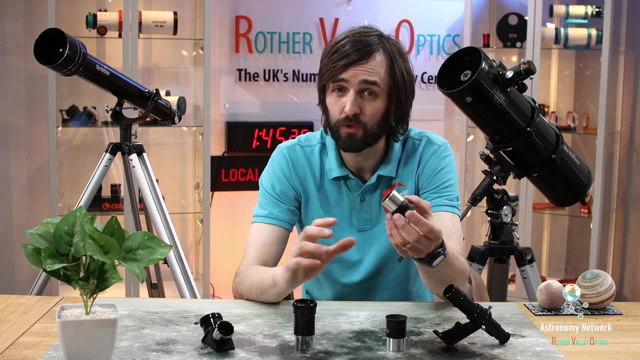 that means is you can purchase eyepieces at a later date to get more or less magnification. now what I would probably recommend is upgrading the 10 mil, maybe going for something with a bit more magnification, something around five or six mil, and maybe the other end of the spectrum. maybe you want to, you know, get. 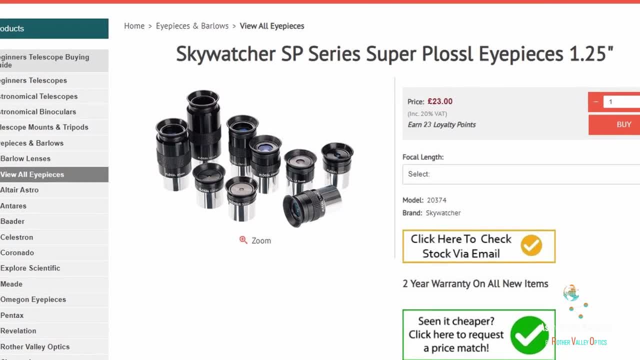 a really wide angle view of the sky. you can get a really wide angle view of the sky, so maybe look at something like a 32 mil now. there's going to be some recommendations on the screen now if you want to have a look at those and they'll. 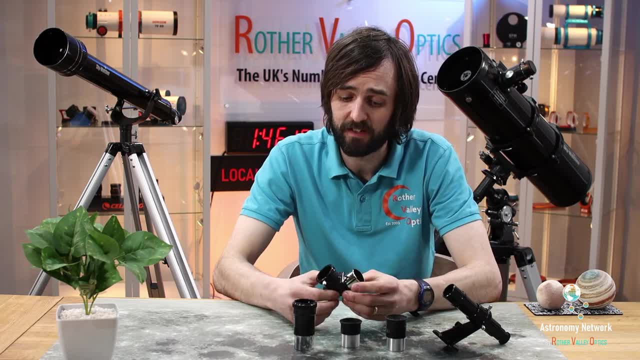 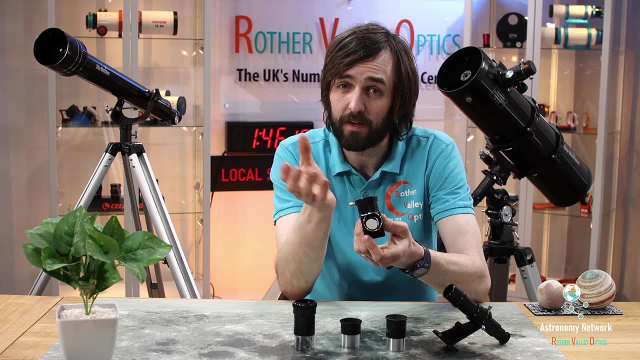 also be linked below. also, if you're going for a refracting lens, I would also consider changing the diagonal that comes with it, and there's nothing wrong with what comes in the box, but everything's going to be inverted with a standard diagonal. what you want to look for is maybe an erecting prism, and that's. 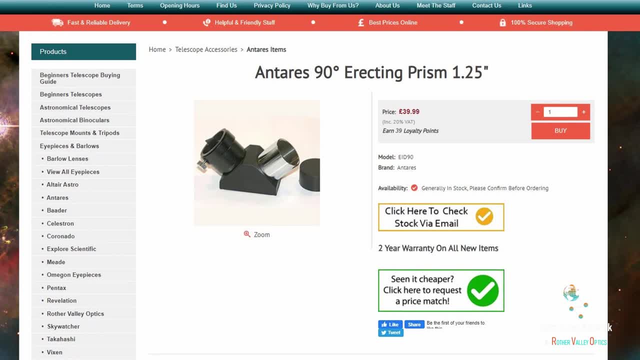 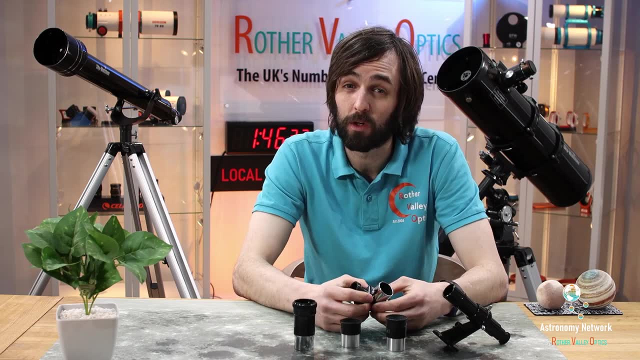 going to be on the screen now. now, what an erecting prism does? it corrects the image. so if you're using it for daytime use, everything's going to be the right right way around. so, yeah, I would highly recommend looking at one of those as well. so that pretty much covers what comes with your scope. but there are a 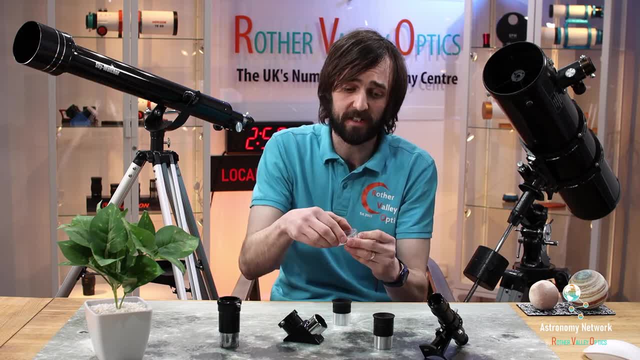 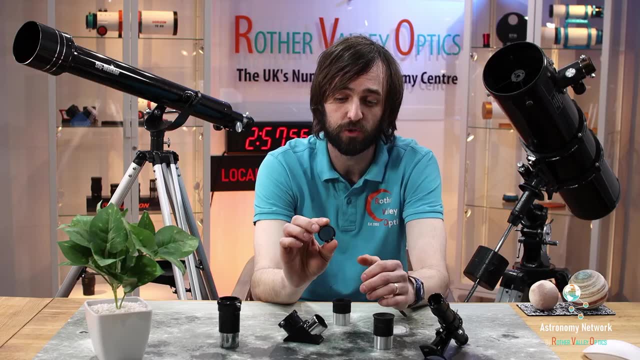 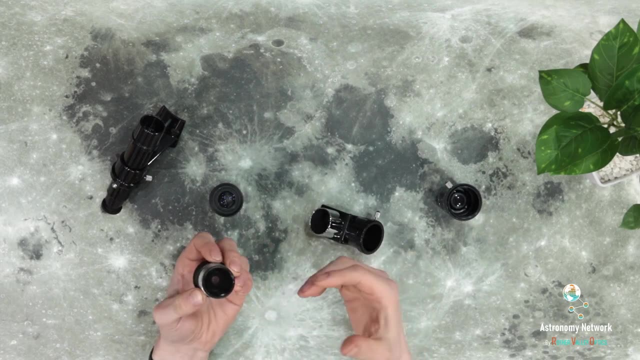 few things we would recommend for a first-time buyer. one of those is a moon filter. now, these are very inexpensive: they only cost 10 pounds. and what it does? it reduces light when looking at bright objects. so, very simply, they just screw onto the bottom of one of the eyepieces and what it does? it reduces. 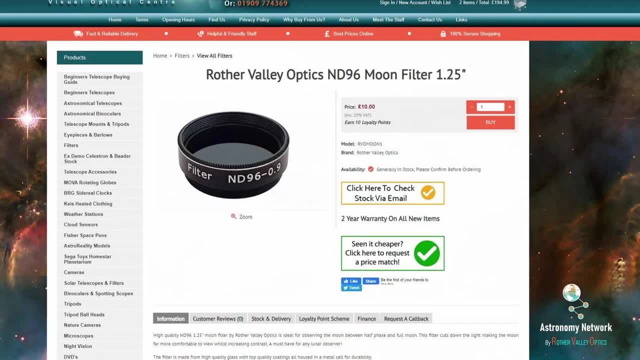 light. if you're looking at the moon, it's going to get rid of the glare, it's not going to be uncomfortable to view and you'll see a lot more detail. you can also use these on planets as well, especially on Jupiter. it's very, very bright, a lot of. 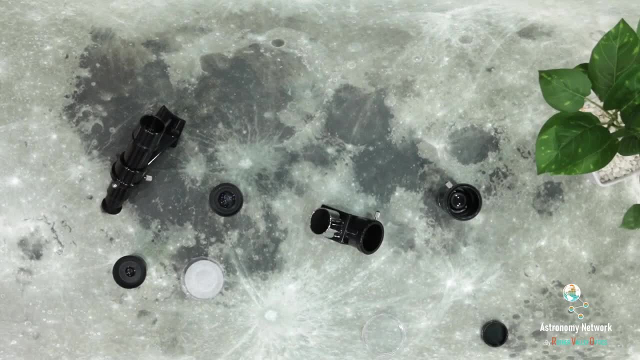 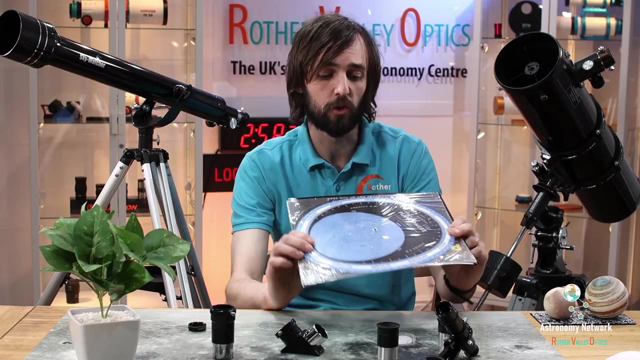 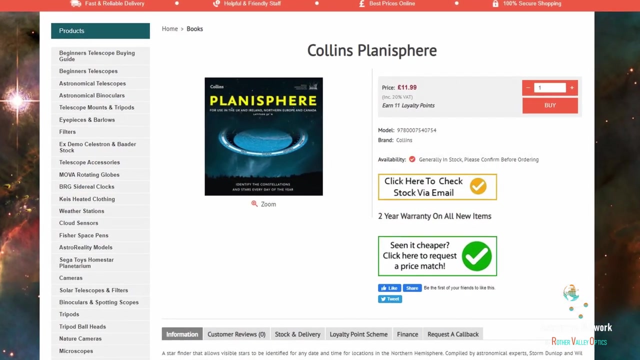 the times, so that will reduce the light there as well. another thing is we do something called a Collins planisphere. now these are very popular for beginner packages. what it does: it will tell you what constellations are visible each night and you rotate it. it's got all the dates. it's basically like a calendar. so 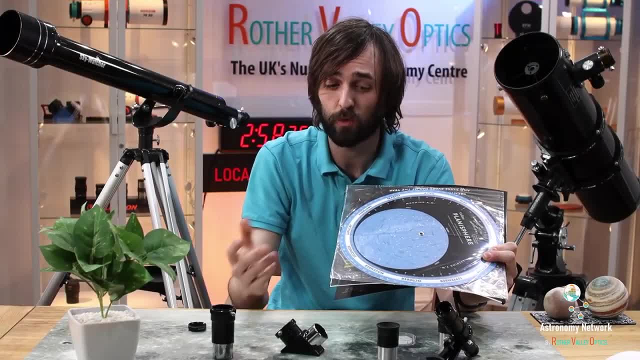 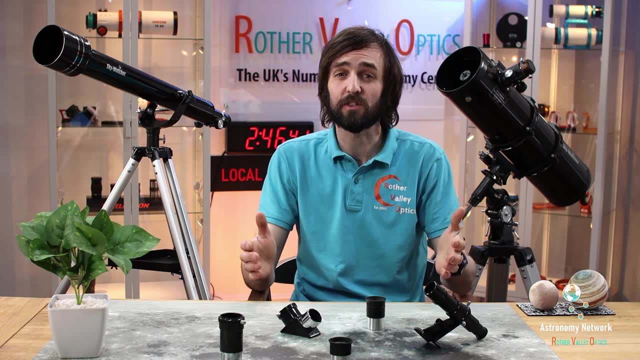 yeah, we would recommend those as well. there'll be links below to both of these, so if you want to check those out, you can find them there. so that pretty much covers all the basics, from a different lenses to different mounts and all the accessories that come with. 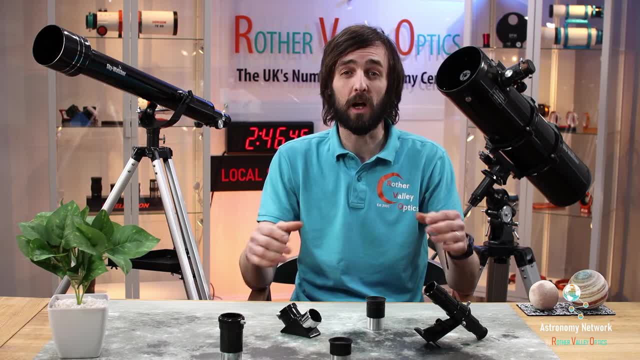 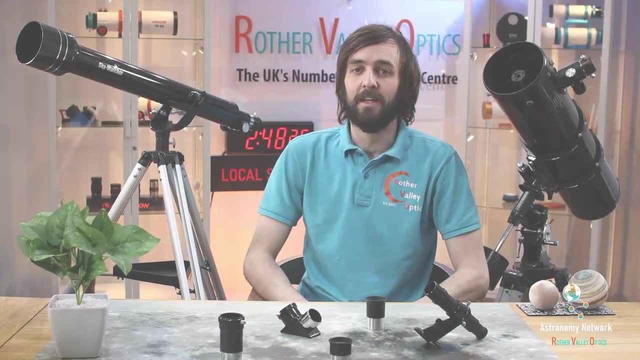 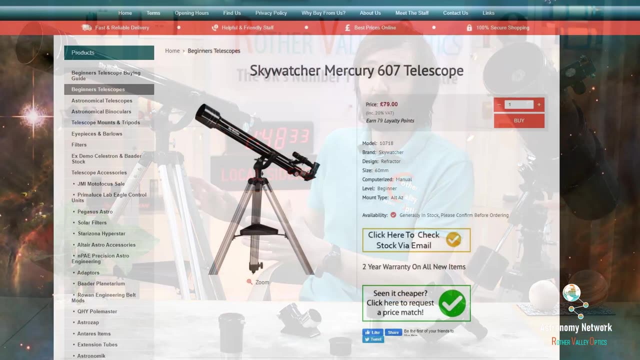 them. so now I want to talk about what telescopes are available and what I would recommend when buying your first scope. so this telescope I've been using as an example is called the Mercury 607. it's made by Skywatcher. now I highly recommend this one if you're buying for a child or anyone who's just starting. 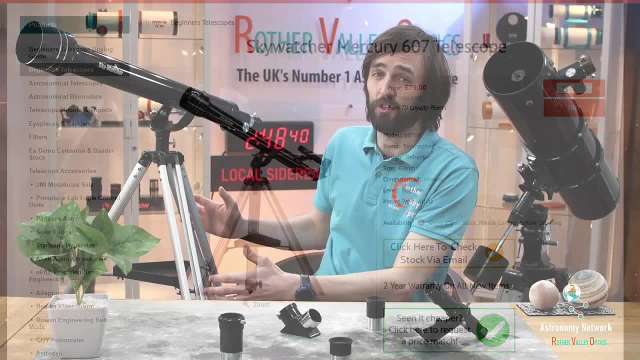 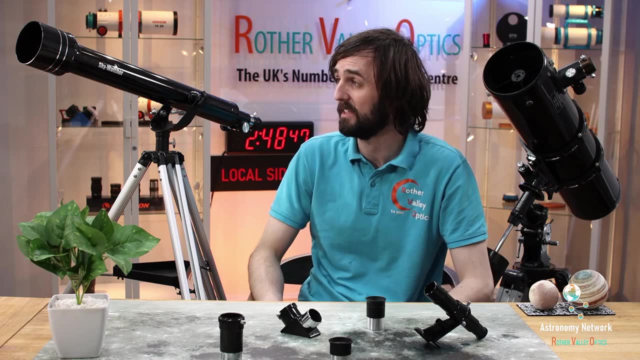 out. really, you know it's not too much money. this entire package costs 79 pounds and that comes with everything. it comes with all those accessories and attention, your scope and your tripod, so for the money it's absolutely fantastic. you can also get a 70 millimeter version as well, so if you're looking for a bit, 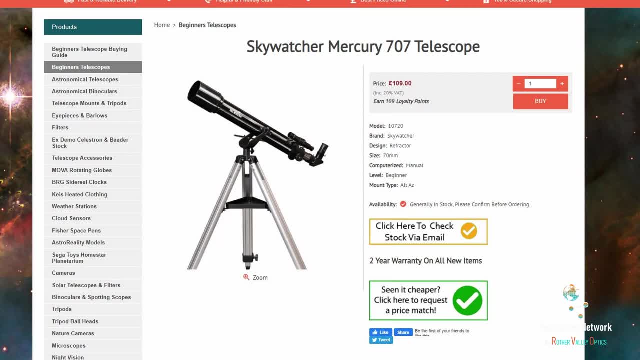 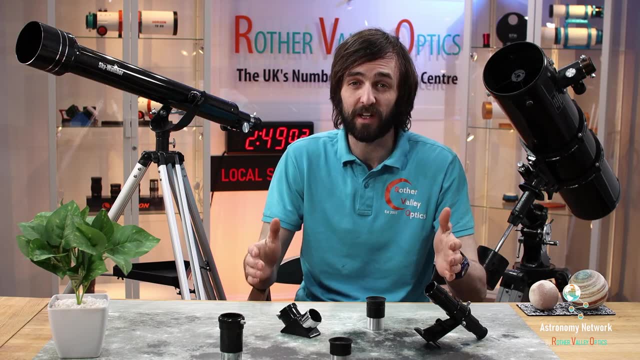 brighter aperture. it might be worth looking at the 70 mil version as well, and that can be picked up on our website for 109 pounds. now, all the links will be below, so if you want to read all the specifications and information, you can follow that link there. now moving on to the reflectors, in my opinion the Skywatch. 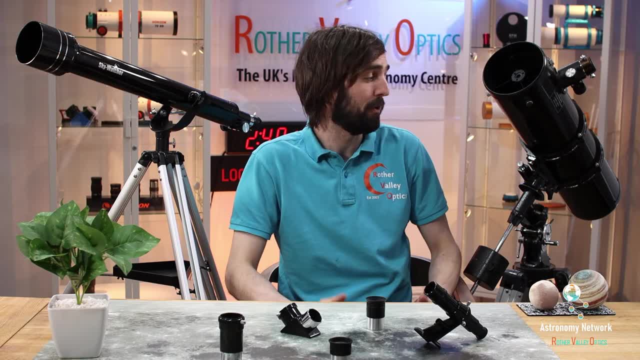 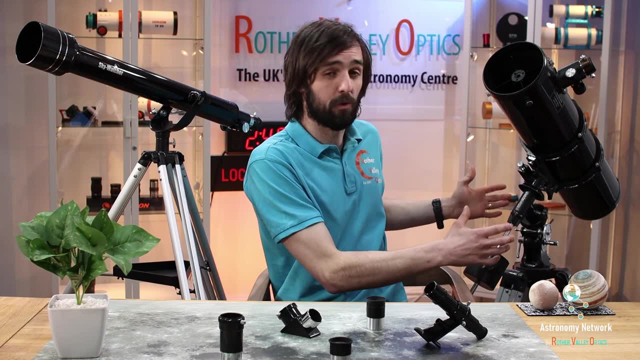 Explorer 130s are pretty much the best bang for your book. you know you get such a big aperture for your money. there's not much else on the market where you get such a big aperture and such a stable and smooth mount for that sort of price. now the one I would normally recommend is 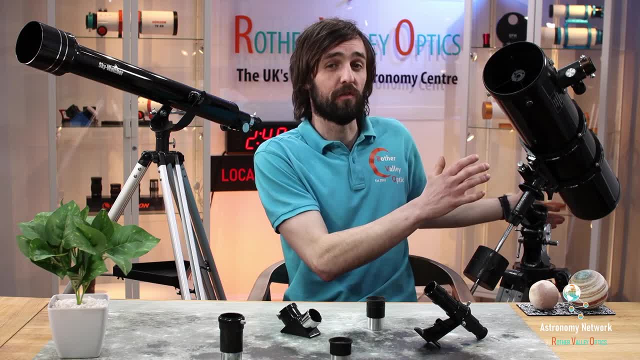 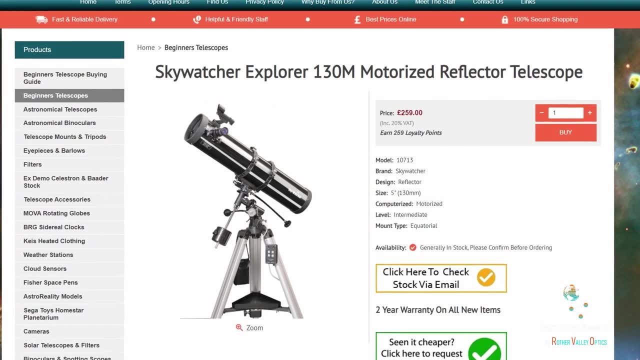 the Explorer 130m. it's the 900 millimeter version of this one, and it also comes with a motor drive, so when you're moving your mount, rather than having to move it manually, you actually control it with motor. now again, that should be on the screen now. links will be below. so if you want, 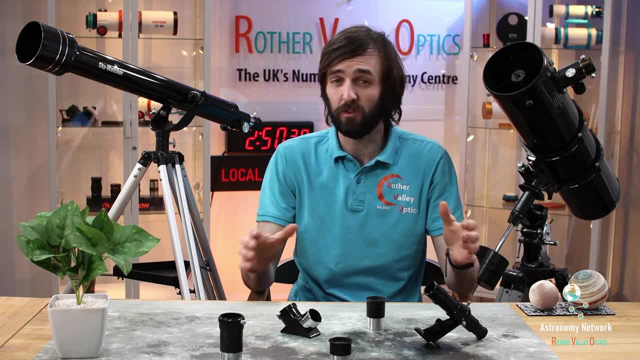 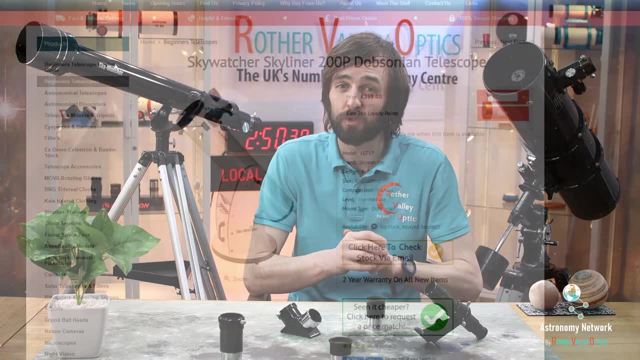 to read all the specifications you can do now. I've only scratched the surface on the types of examples. another good range that we recommend are the Skywatcher Dobsonians- they're very popular at the moment- and also maybe look at some of the go-to telescopes. now I'll probably be making 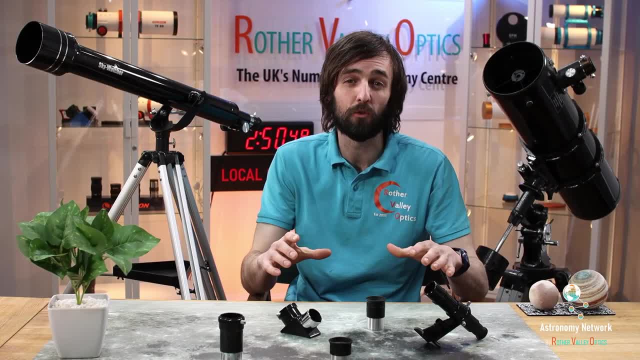 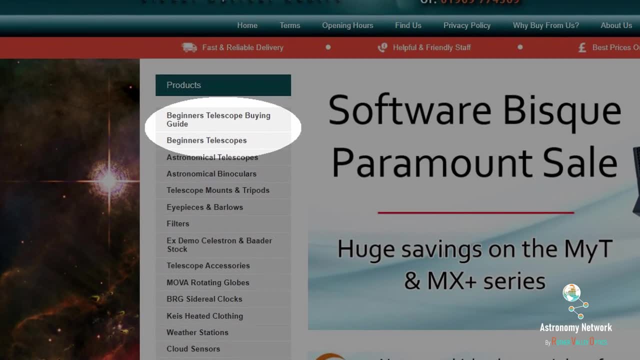 another video specifically on the go-tos because they are a little bit more in depth. there will also be a link below taking you to all of our beginner telescopes so you can see the full range on there. if you've got any questions or you need any advice about any of the beginner,